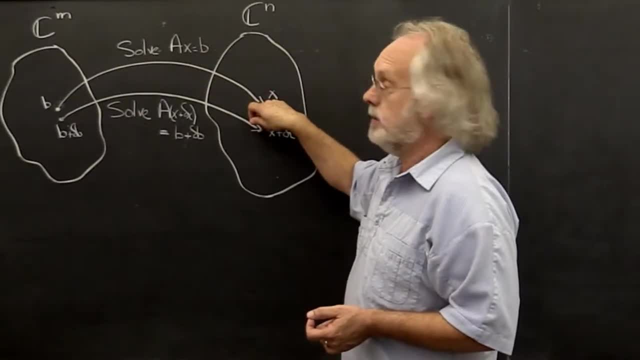 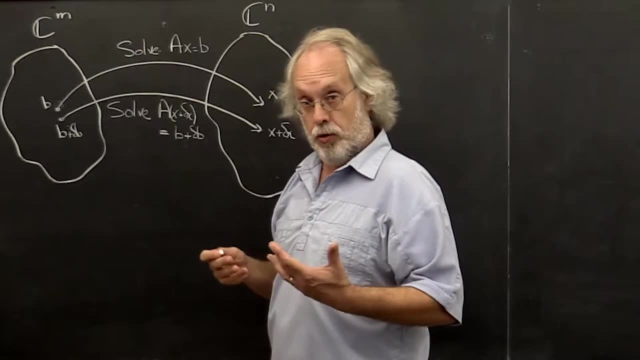 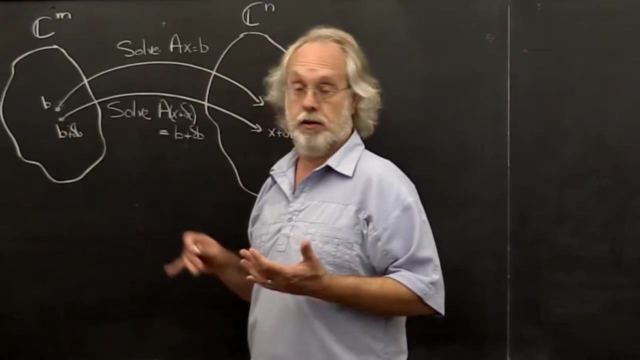 gives you an output vector x, the solution. What if you'd make a small change to b? For example, what if how you measured the right-hand side b wasn't all that simple, Accurate, So you know that there's a little bit error in it? Or what if you started? 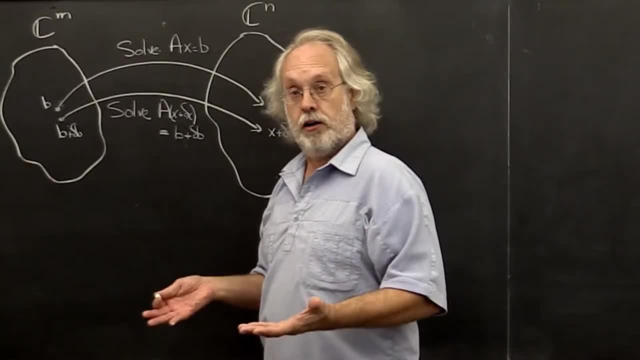 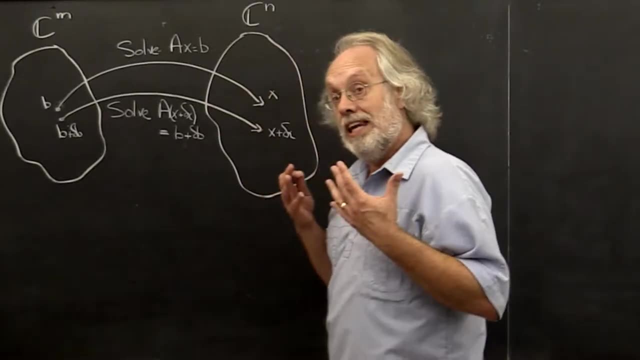 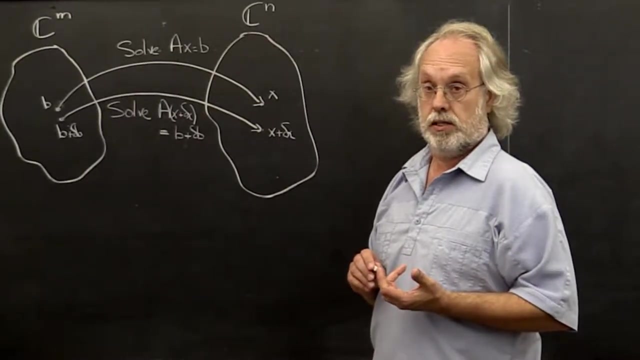 with a vector. you stored it in a computer and I don't know if error happens when you store it. A small error would occur, Obviously. what you would like is for there to be a small error in the solution as well- Small, well, you know how. 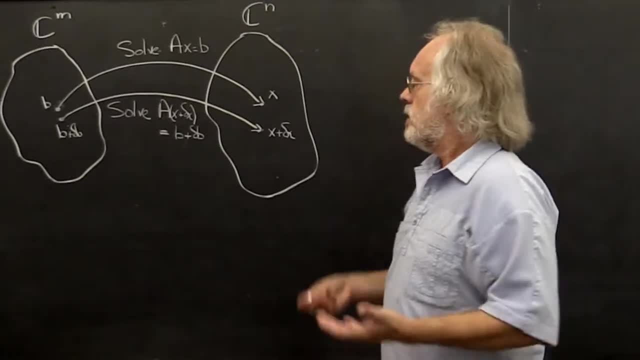 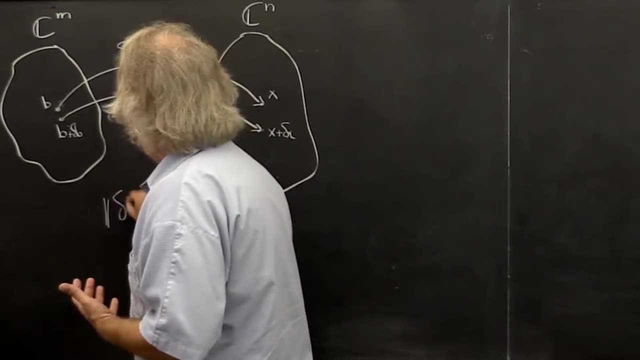 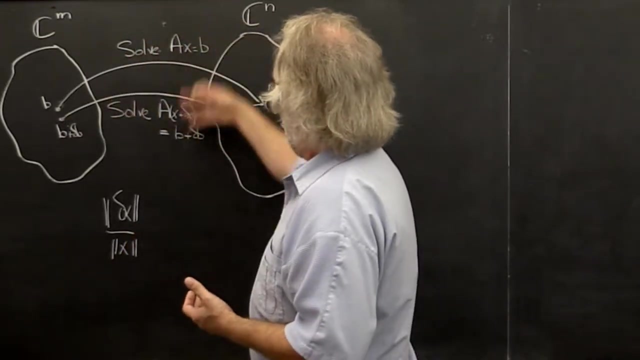 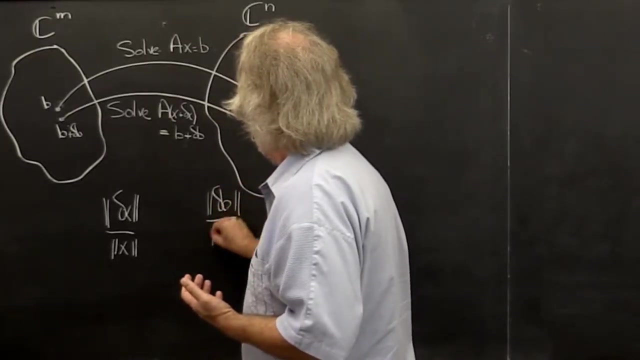 to measure small now We use vector norms, But really we are interested in relative error. We're really interested in the change in x relative to x that results when you do these two computations And you want to compare that to the relative error in b. Now let me take a timeout and 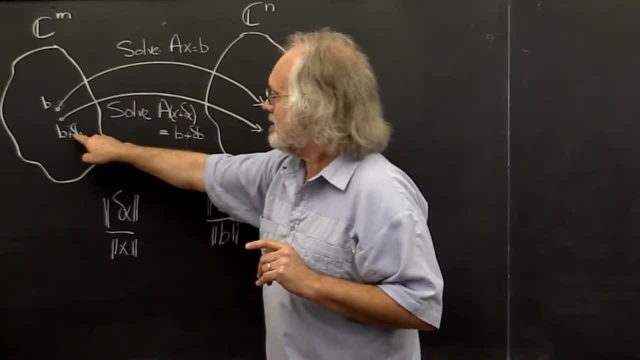 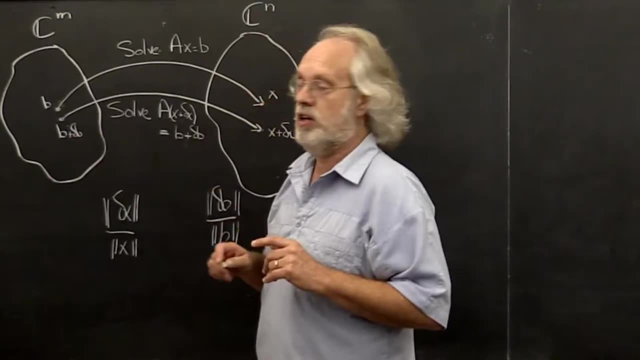 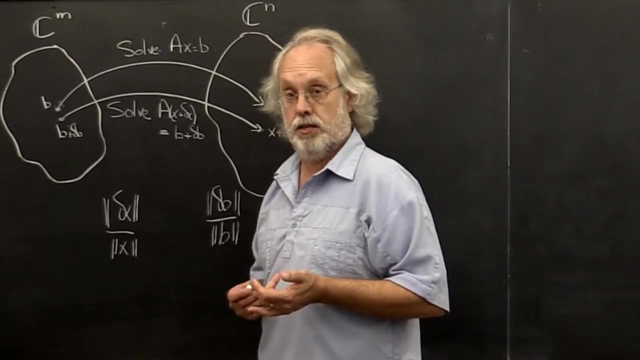 just point out this is not delta times beta. In other words, it's not a scalar times the vector B. I'm purposely trying to make the Delta and the B touch to indicate that this is just a label for the vector that represents the change in the vector B. So let's try to keep track. 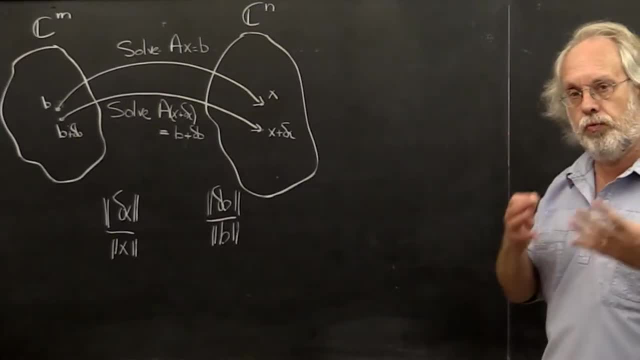 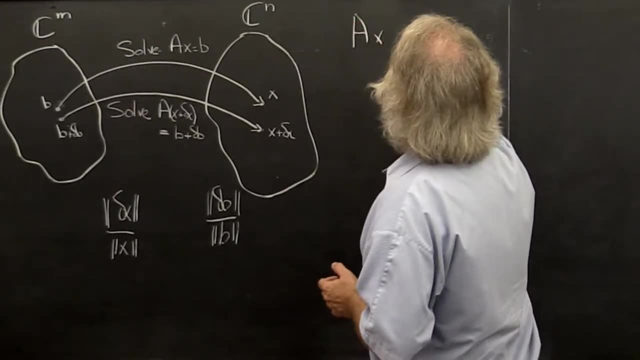 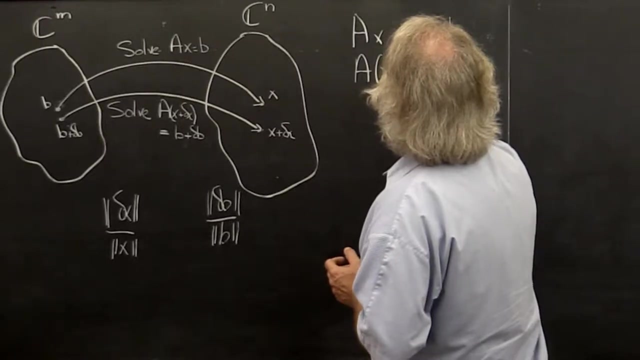 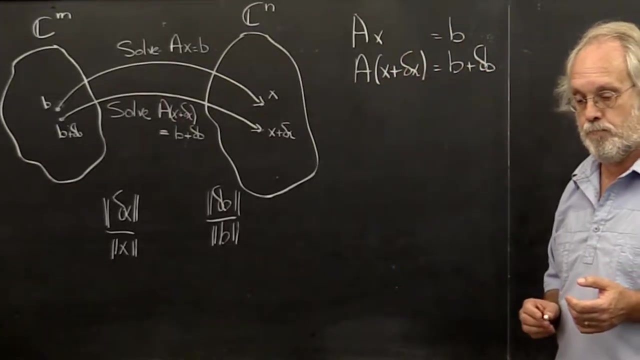 of that. Sometimes they may not quite touch, but hopefully you can stick with me. Now, what do we know? We know that A times x is equal to B, And we also know that A times x plus Delta x is equal to B plus Delta B. right, We know that, matrix. 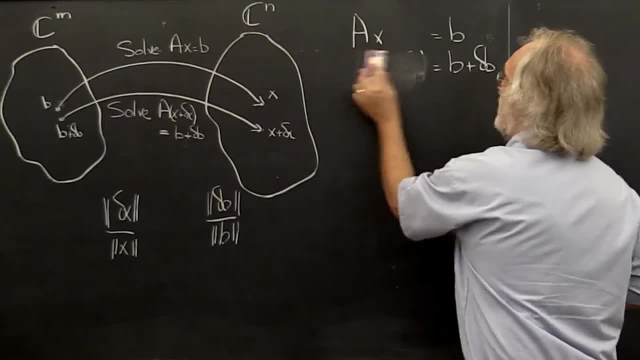 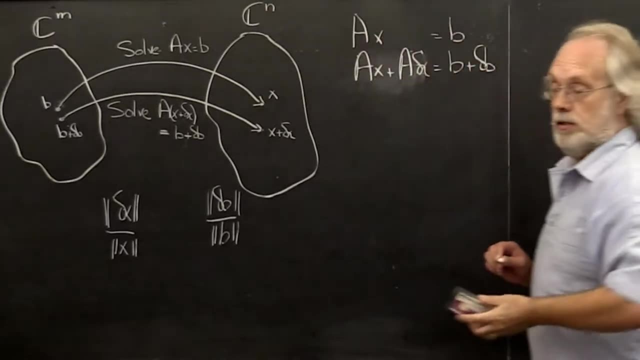 vector multiplication distributes. So we can replace this by A times x plus A times Delta x Right, And then we can take the first equation and subtract it off the second. alright, echt mensen, om legen das schapen untuk das schwerming feminollowd. 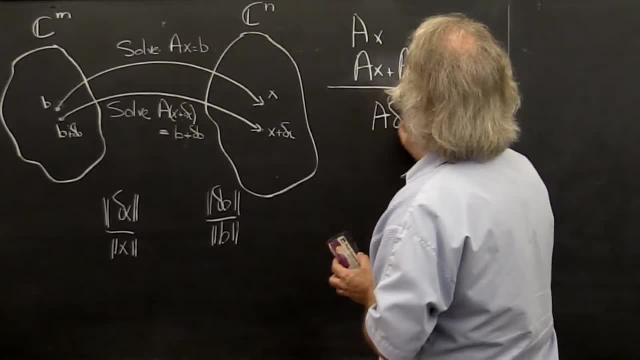 зак servers, And then we can take the first equation and subtract it off the second, each one of them byuous levels, And that's gonna give us an answer to, of course, equation and say, oh, that leaves us with a times: delta x is equal to delta b. So 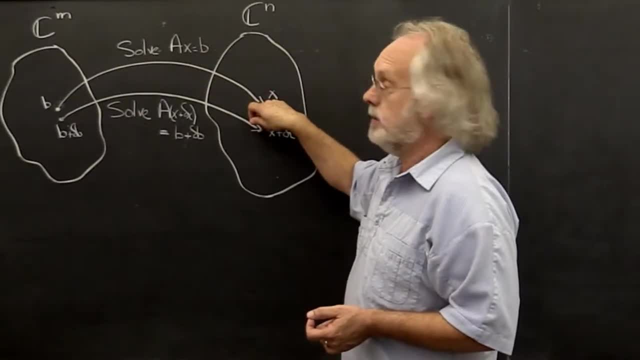 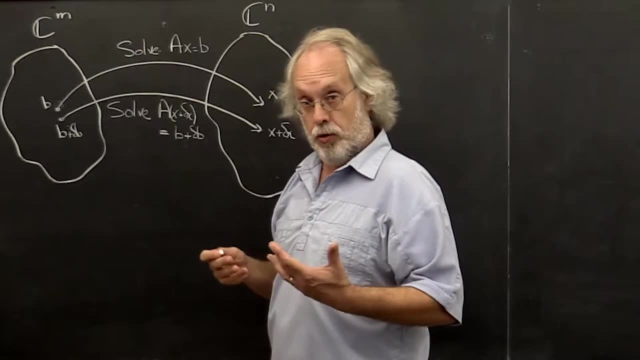 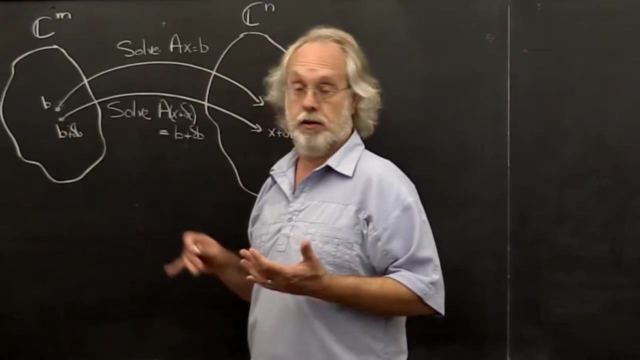 gives you an output vector x, the solution. What if you'd make a small change to b? For example, what if how you measured the right-hand side b wasn't all that simple, Accurate, So you know that there's a little bit error in it? Or what if you started? 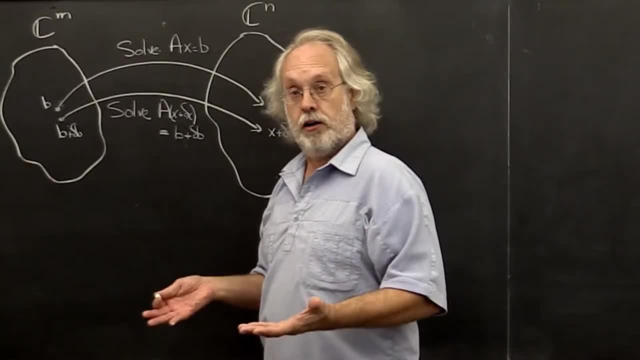 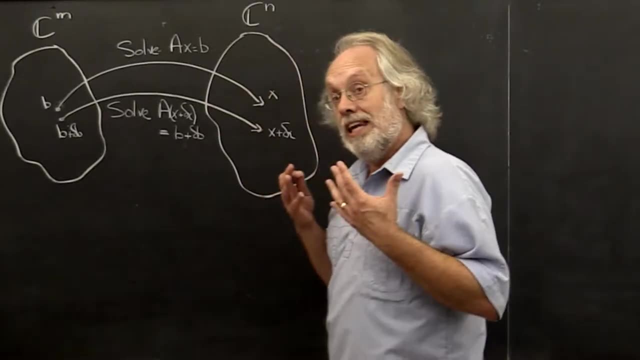 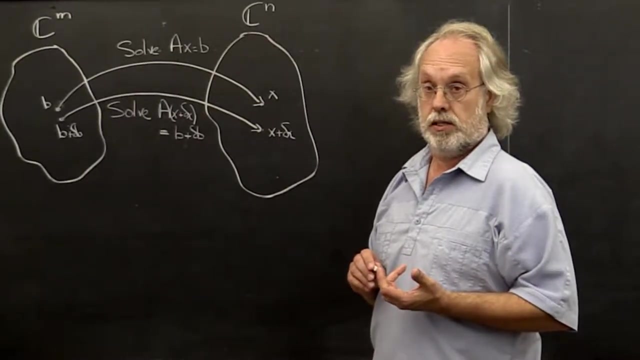 with a vector. you stored it in a computer and I don't know if error happens when you store it. A small error would occur, Obviously. what you would like is for there to be a small error in the solution as well- Small, well, you know how. 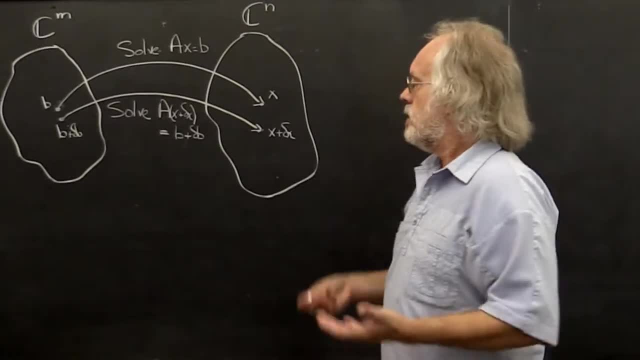 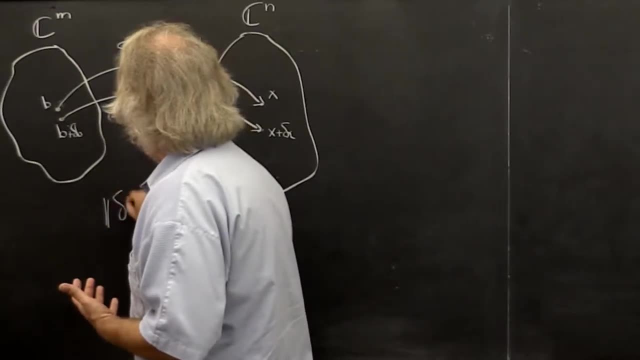 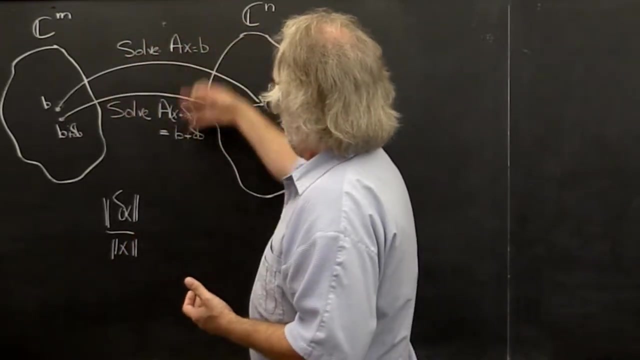 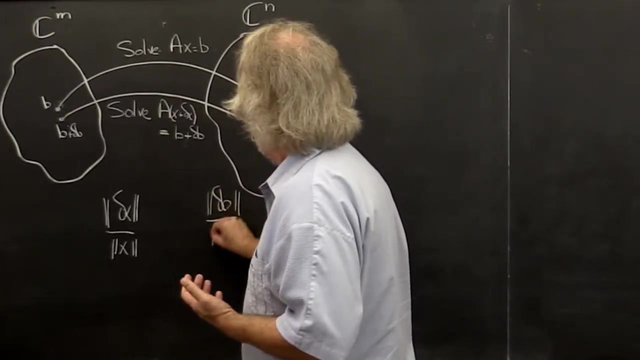 to measure small now We use vector norms. But really we are interested in relative error. We're really interested in the change in x relative to x that results when you do these two computations And you want to compare that to the relative error in b. Now let 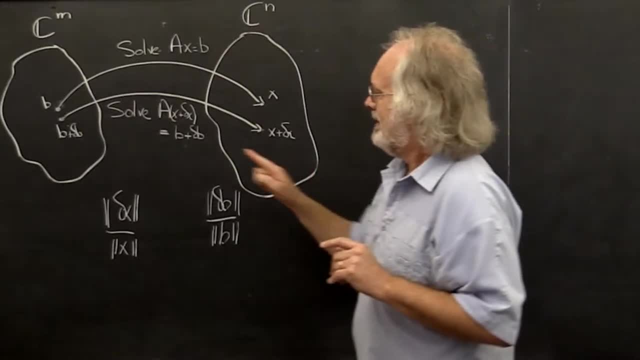 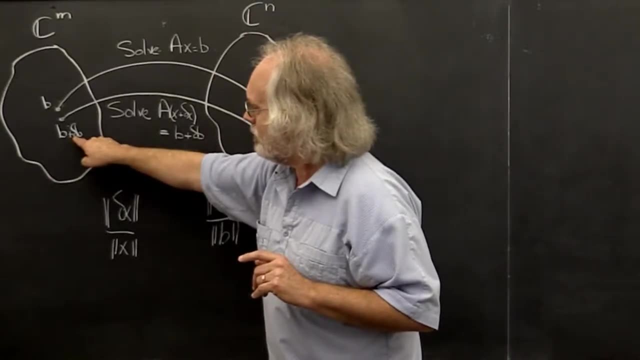 me take a timeout, And so just point out: this is not delta times b, This is a b. In other words, it's not a scalar times the vector b. I'm purposely trying to make the delta and the b touch to indicate that this is just a label for. 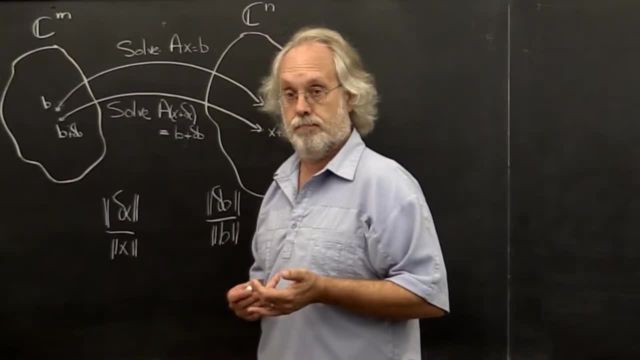 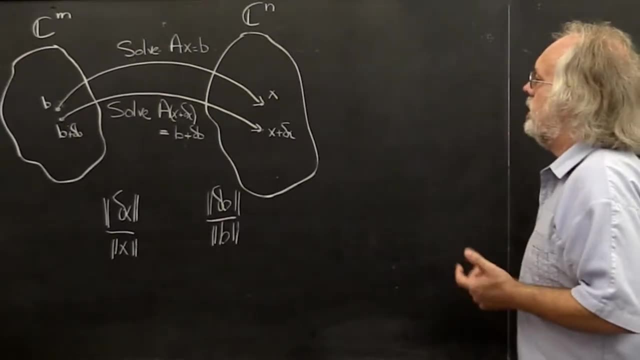 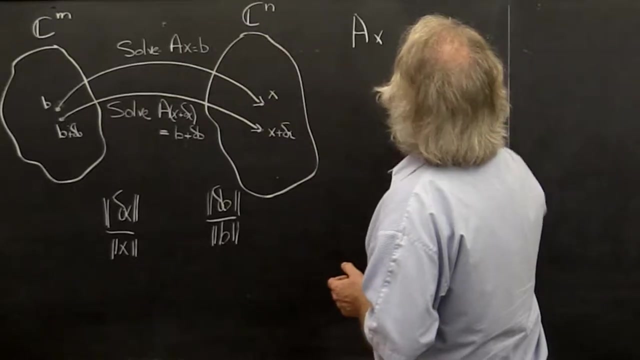 the vector that represents the change in the vector b. So let's try to keep track of that. Sometimes they may not quite touch, but hopefully you can stick with me. Now, what do we know? We know that a times x is equal to b, And we also know that a- 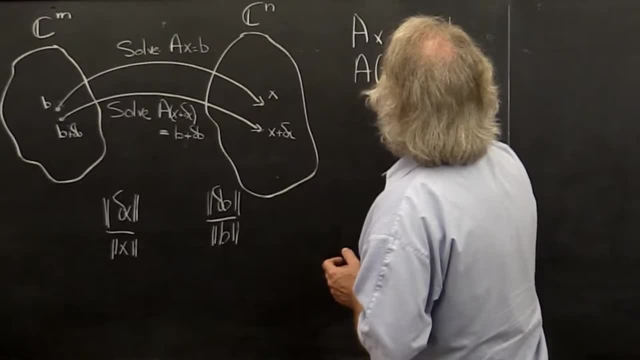 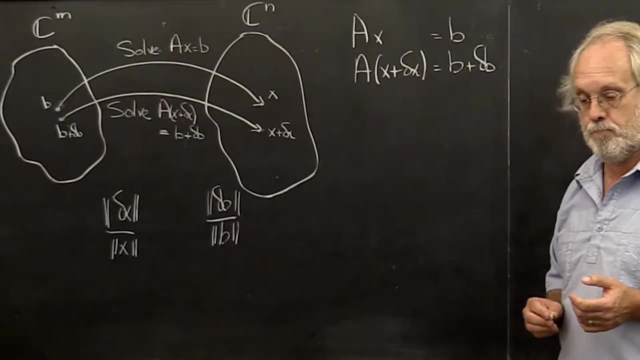 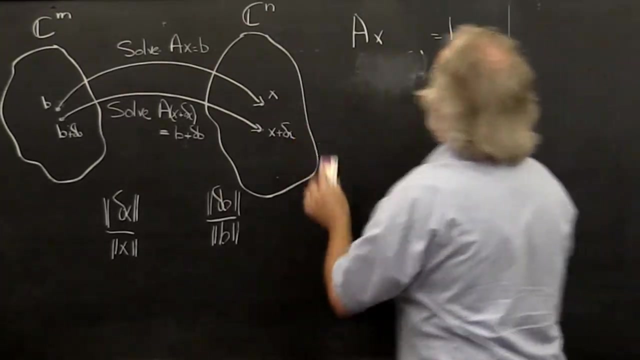 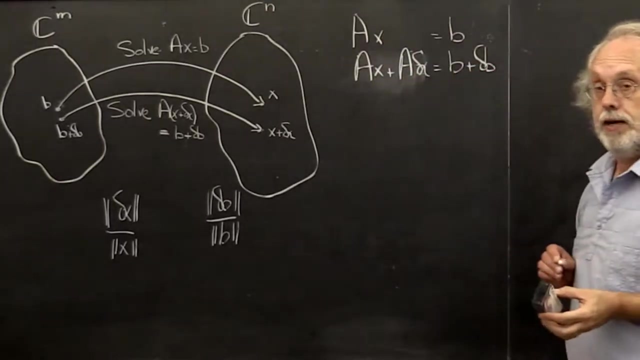 times x plus delta x is equal to b plus delta b. alright, We know that matrix vector multiplication distributes, so we can replace this by a times x plus a times delta x. alright, And then we can take the first equation and subtract it off. 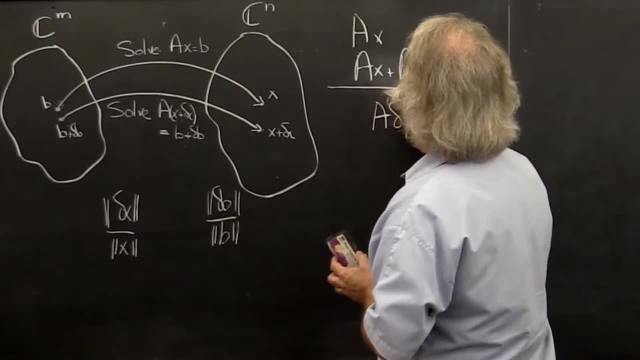 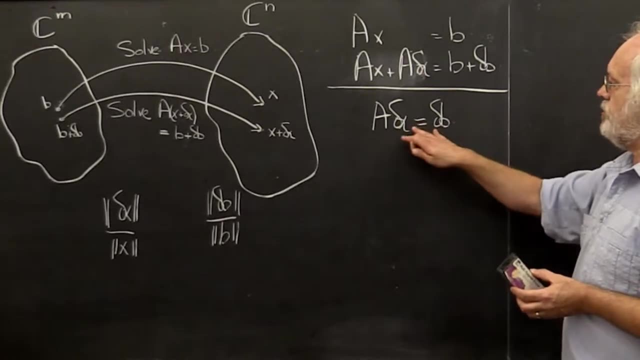 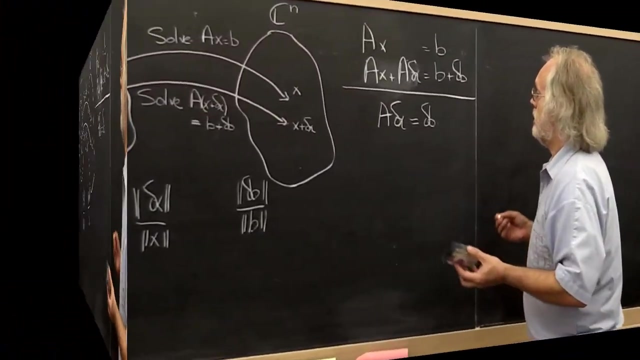 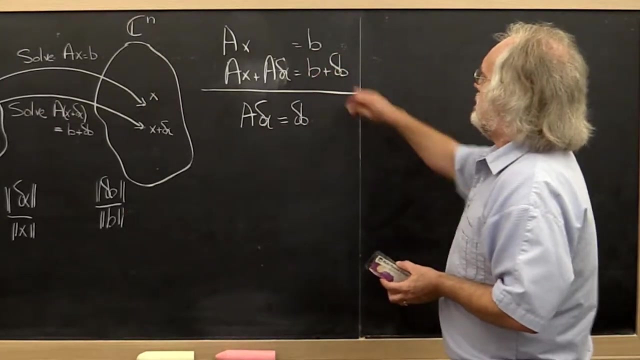 the second equation, Thank you very much and say: oh, that leaves us with A times: delta x is equal to delta B, So there's this nice relationship between the error that was introduced and the error in the solution. All right, Now we want to start taking some norms, And to do that we 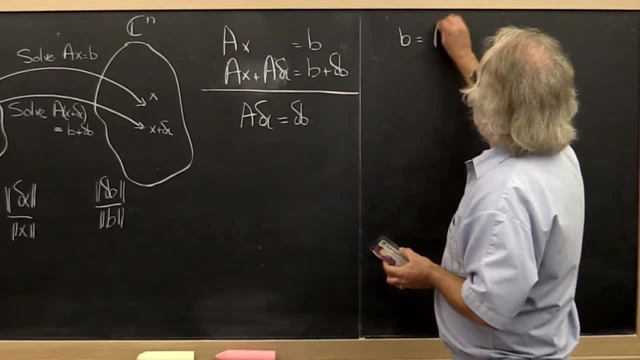 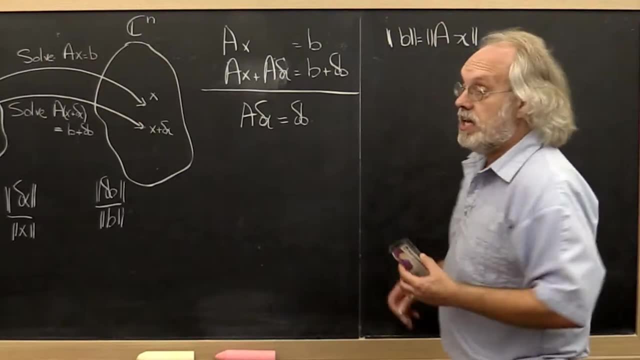 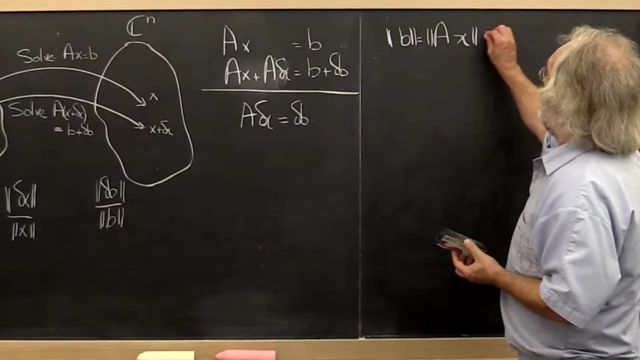 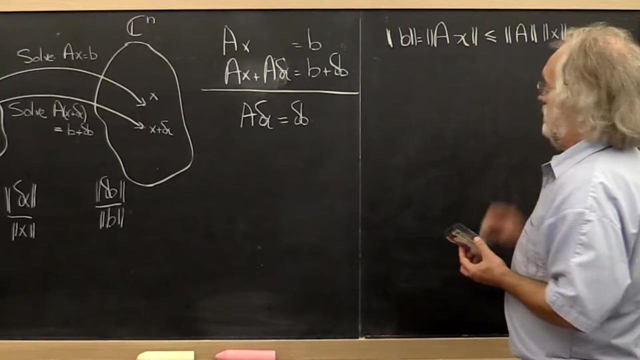 start with this And we rewrite it as B is equal to A times x, so that we can take the norm on both sides. And then if we used an induced matrix norm, then we know that this is less than or equal to the norm of A times the norm of x. All. 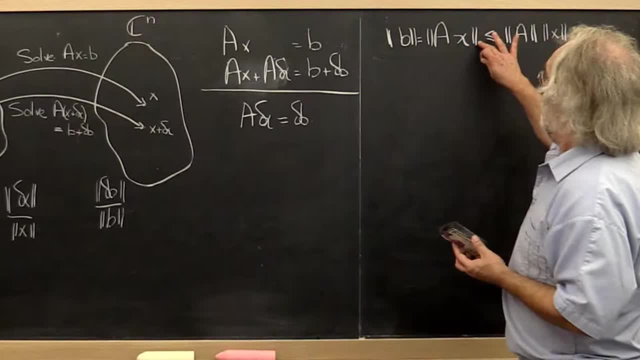 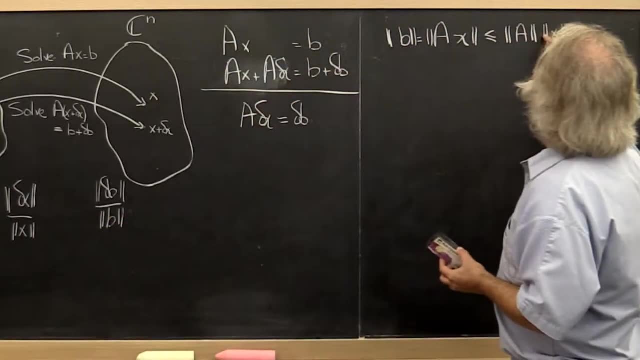 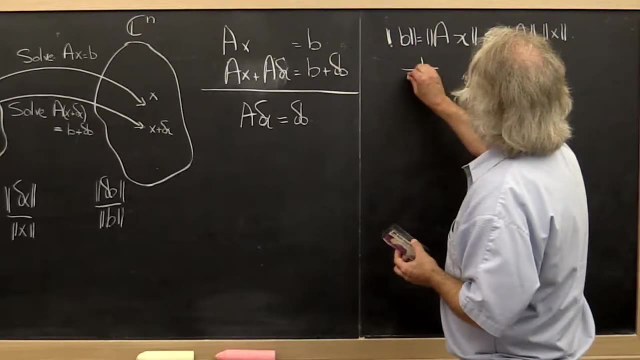 right. We can actually rearrange this to get something that looks like it might help us here by saying: let's bring the norm of x to the left, the norm of B to the right and rewrite this as 1 over. the norm of x is less than or equal to the norm of A times. 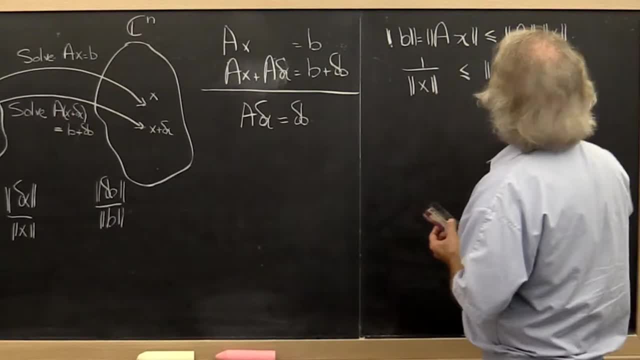 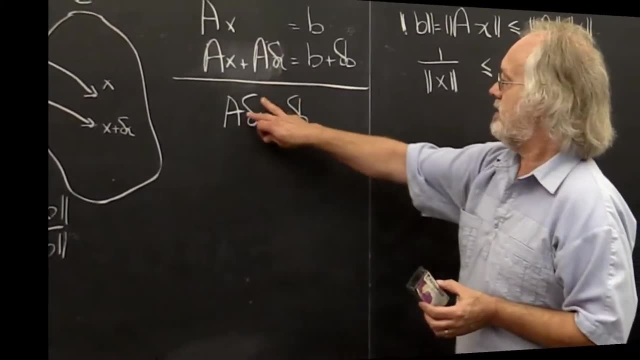 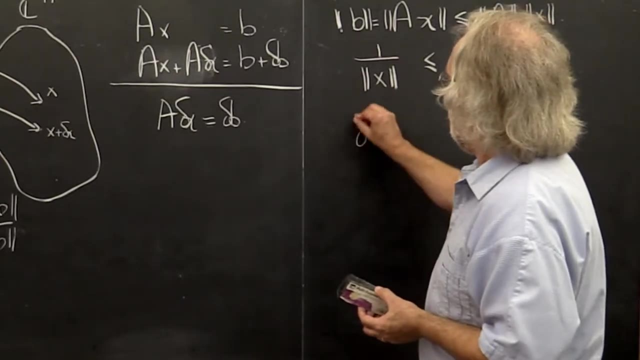 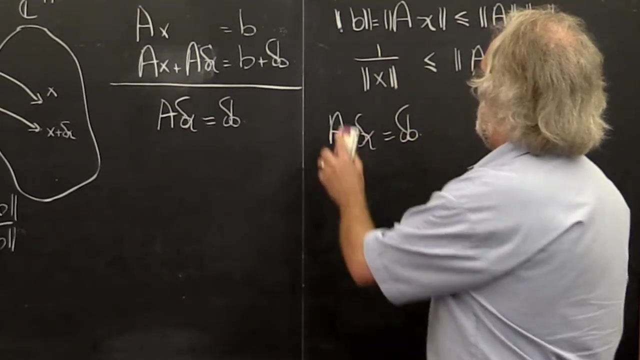 1 over the norm of B. That puts us partially towards this right here. All right. Now we need to somehow relate delta x and delta B the norms, And for that we're actually going to rewrite A times: delta x is equal to delta B, as delta x is. 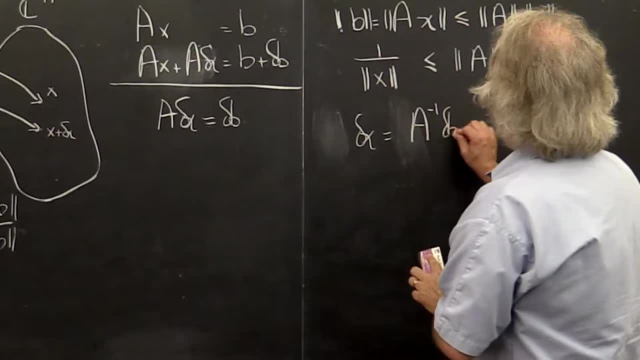 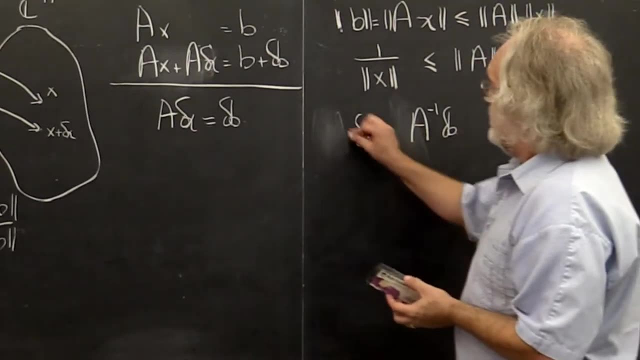 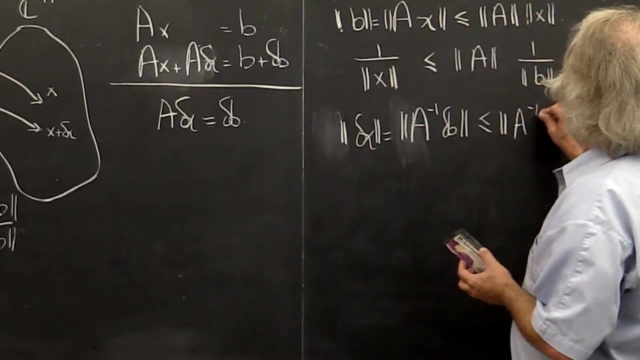 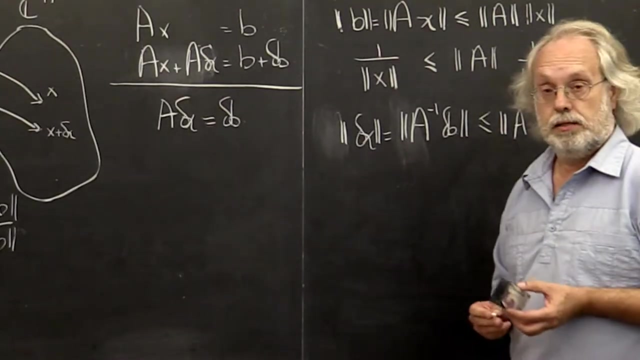 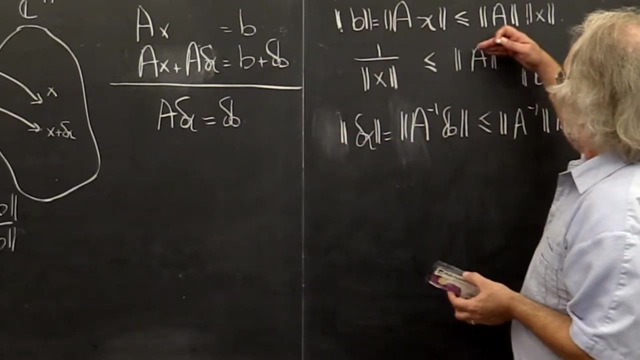 equal to A inverse times delta B. We can do that because we assume that A was nonsingular and therefore we know it has an inverse matrix. Then we can take the norm of that And we can bound that by the norm of A inverse times the norm of delta B. All right, Now multiply this times this on the left and this times this on the right, we get. 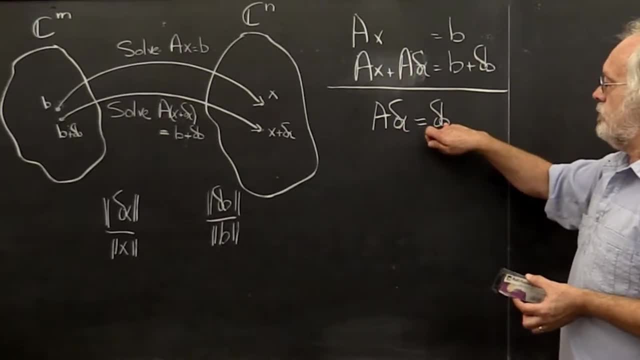 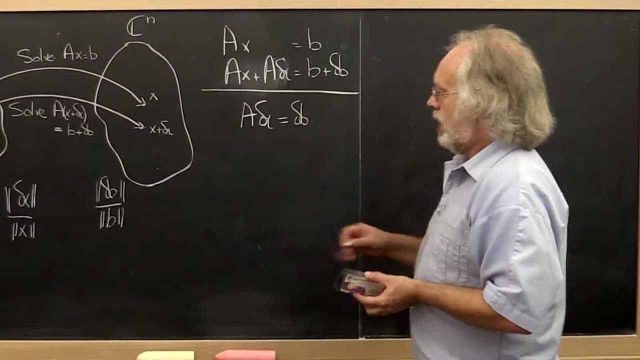 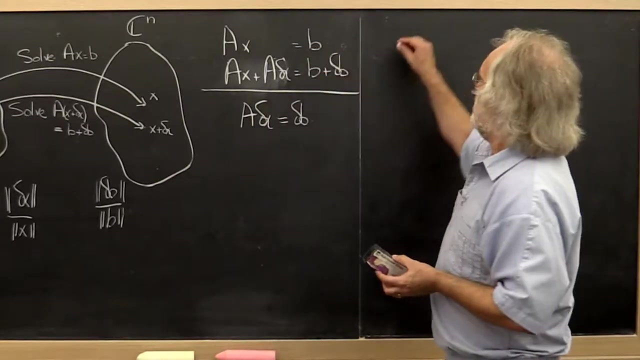 there's this nice relationship between the error that was introduced and the error in the solution. Alright, now we want to start taking some norms And to do that, we start with this and we rewrite it as b is equal to a times x, so 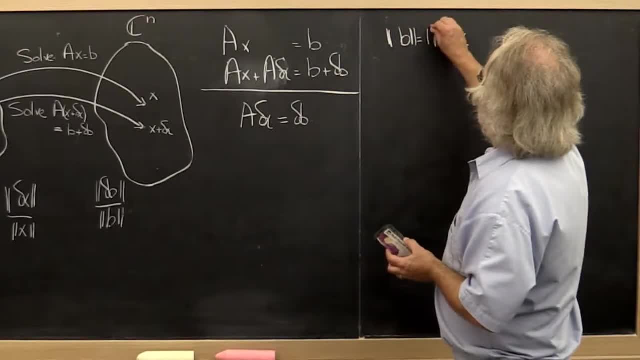 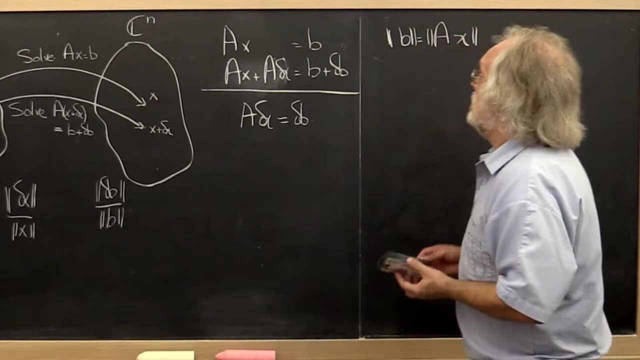 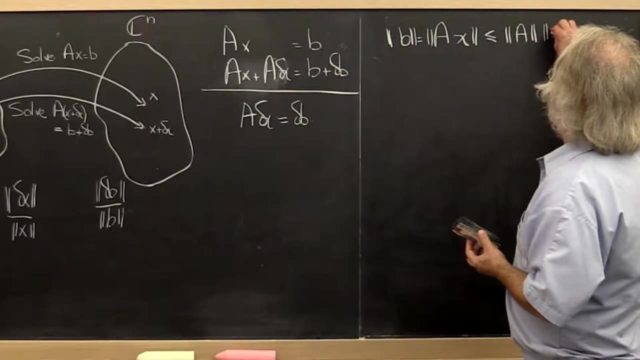 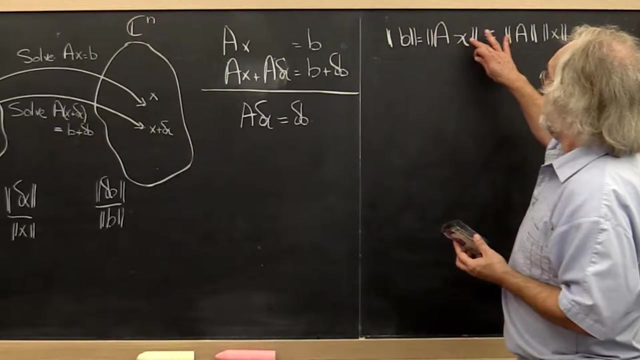 that we can take the norm on both sides, And then if we used an induced matrix norm, then we know that this is less than or equal to the norm of a times the norm of x. Alright, Hmm, We can actually rearrange this to get something that looks like it might help. 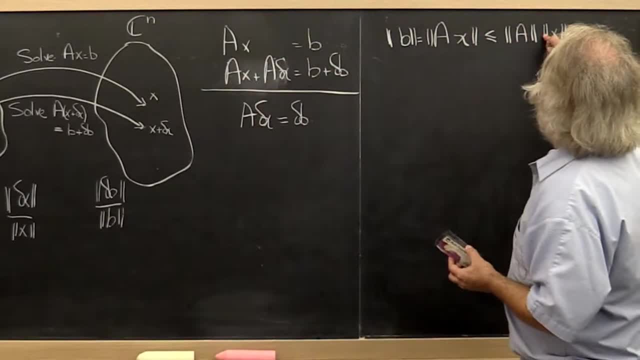 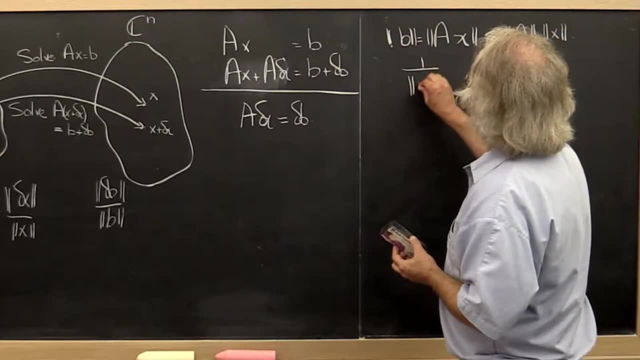 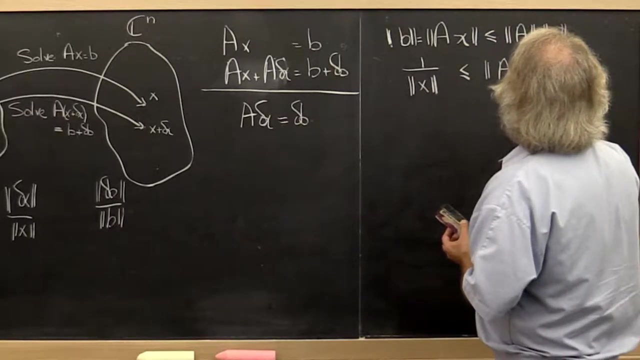 us here by saying: let's bring the norm of x to the left, the norm of b to the right and rewrite this as: 1 over the norm of x is less than or equal to the norm of a times 1 over the norm of b. That puts us partially towards this. 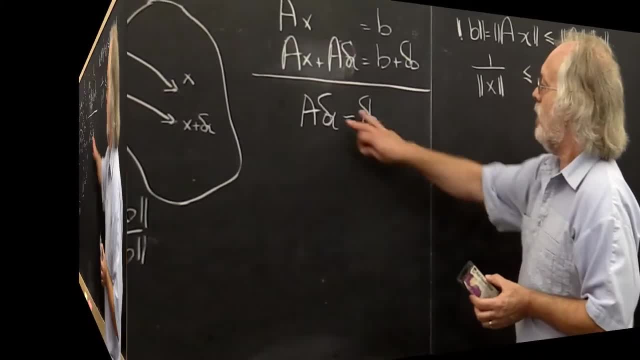 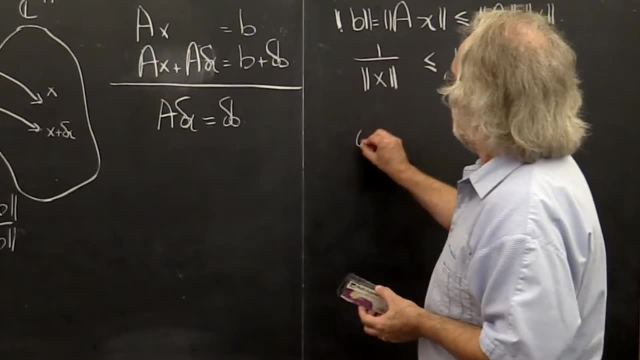 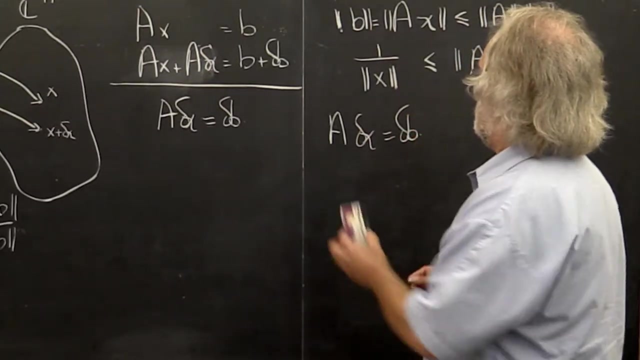 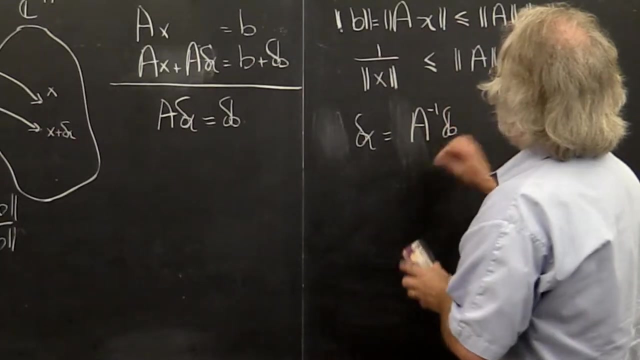 right here. Alright, Now we need to somehow relate delta x and delta b, the norms, And for that were actually going to rewrite a times delta x is equal to delta b, as delta x is equal to a inverse times delta b. We can do that because we assume 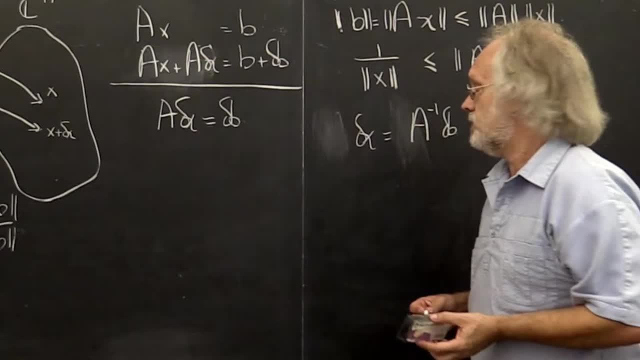 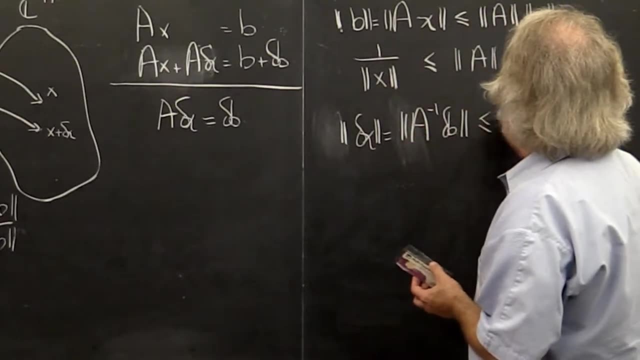 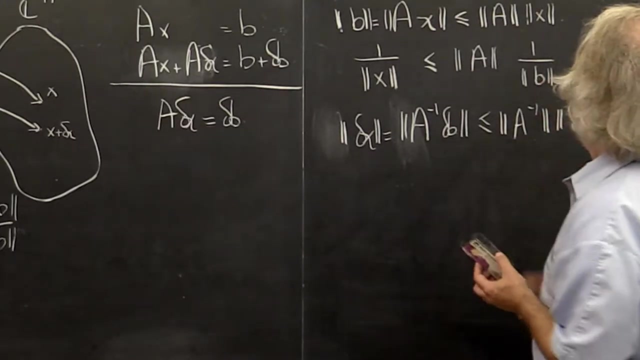 that a was non-singular and therefore we know that it has an inverse matrix. Then we can take the norm of that, then we can take the norm of that and we can bound that by the norm of A inverse times the norm of delta B. 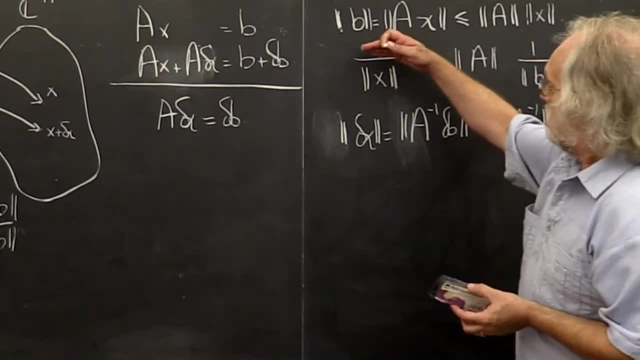 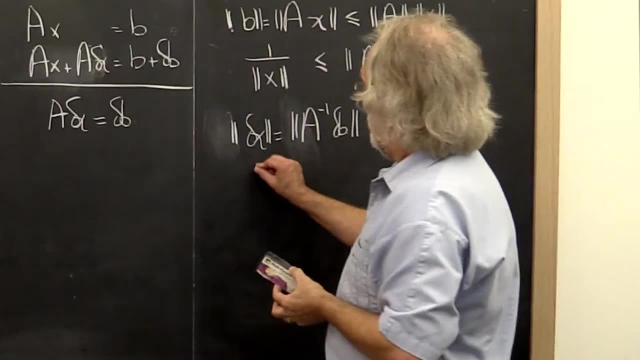 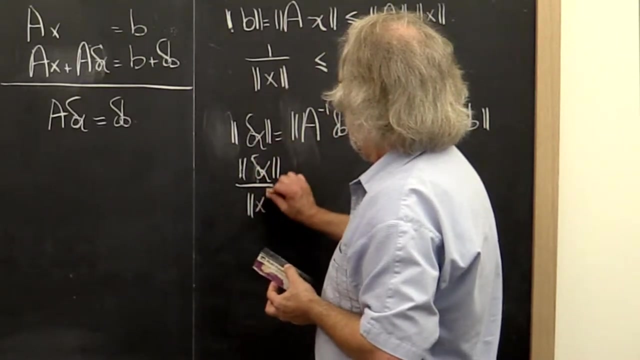 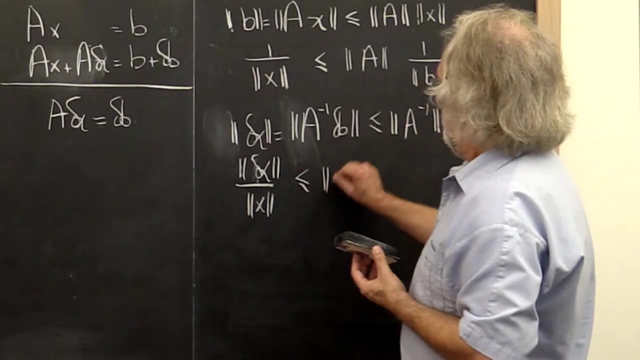 All right Now multiply this times this on the left and this times this on the right. We get one. we get delta x over x. Well, the norm of delta x over x, the relative error in x is bounded by the norm of A. 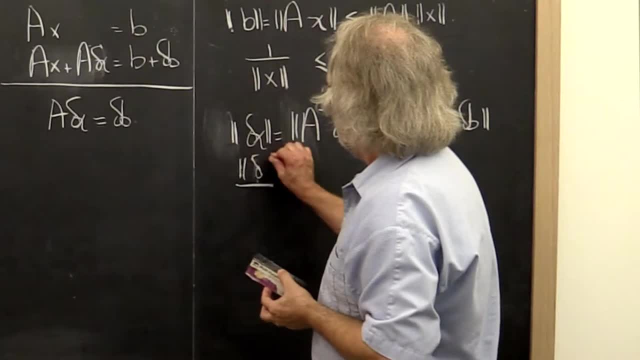 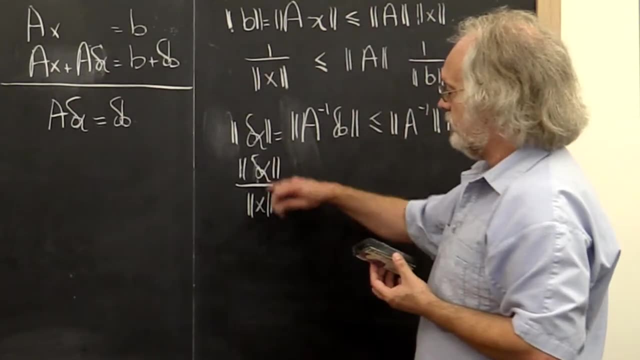 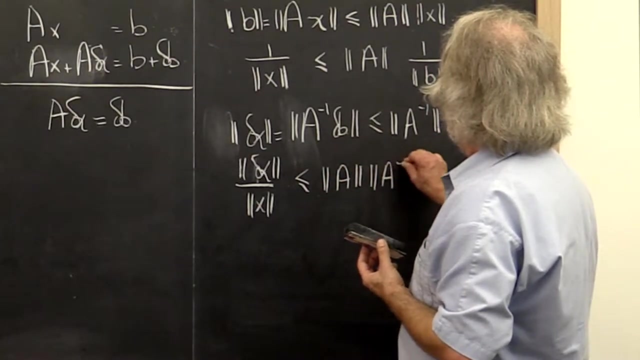 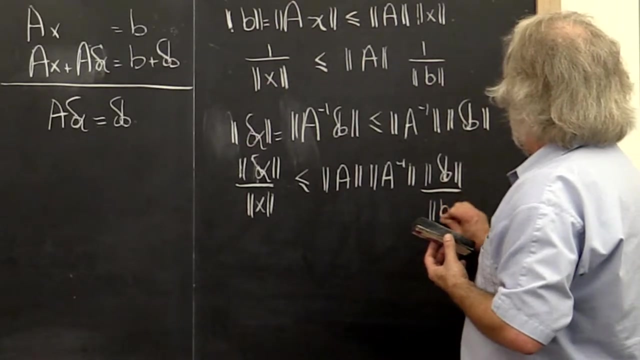 one we get delta x over x. Well, the norm of delta x over x, the relative error in x, is bounded by the norm of A times the norm of A inverse times delta B, the relative error in B. All right, So we now have answered our question. 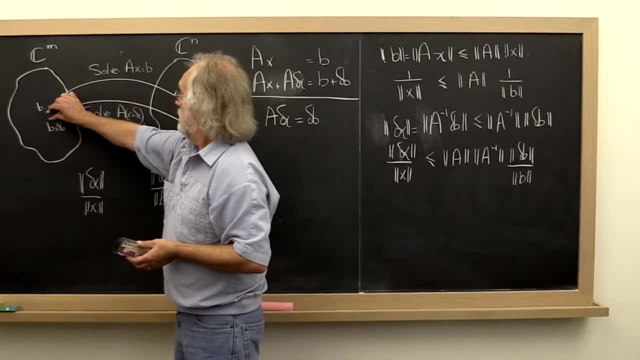 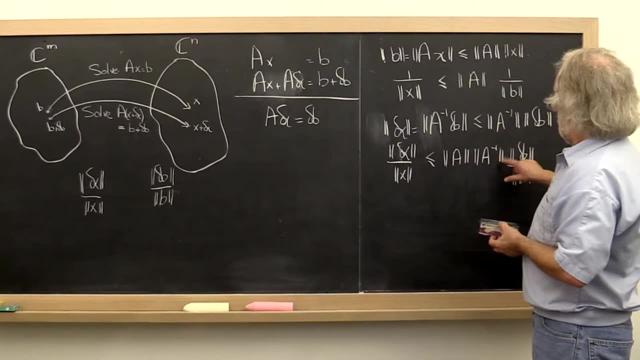 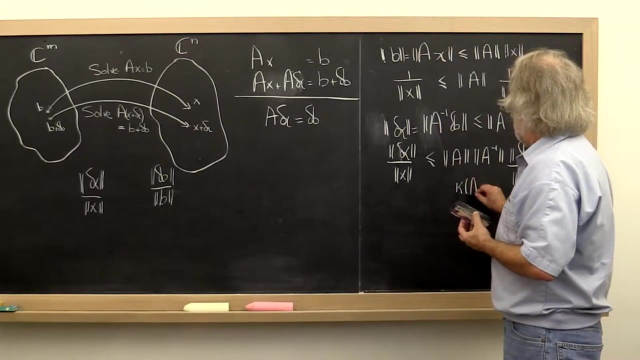 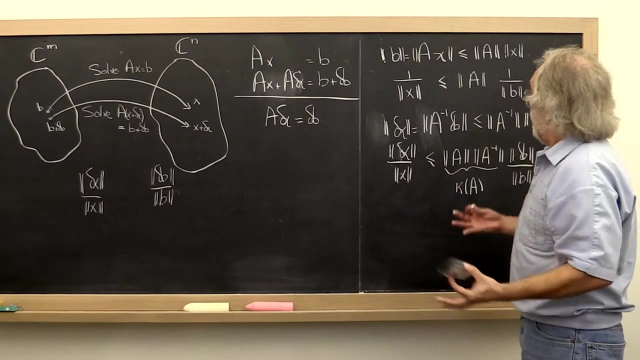 Okay, So we now have answered our question. The small error in B can be amplified no more than this quantity right here, which we call the condition number of matrix A. Obviously, this condition number depends on which norm you chose. Now, when we talked about induced matrix norms, we saw: 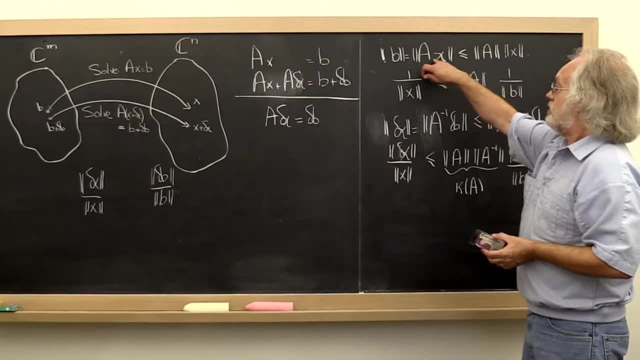 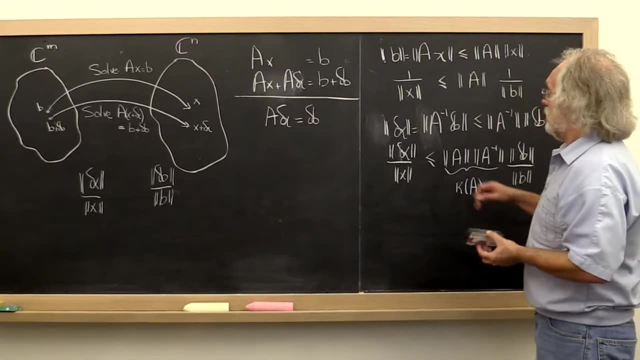 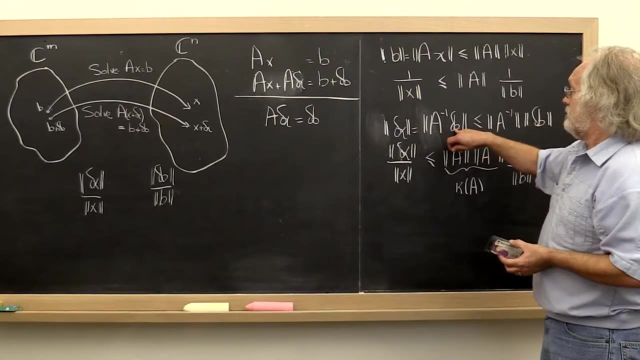 that there is a vector x, such that the norm of A times x is equal to the norm of A times the norm of x. And we saw similarly that there is a choice for delta B, such that A inverse times delta B in norm is equal to the norm of A inverse times the norm of delta B. 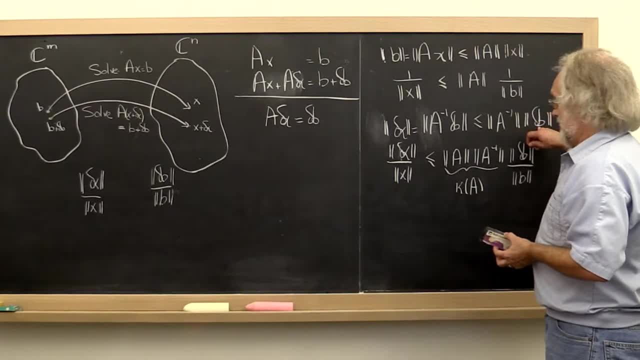 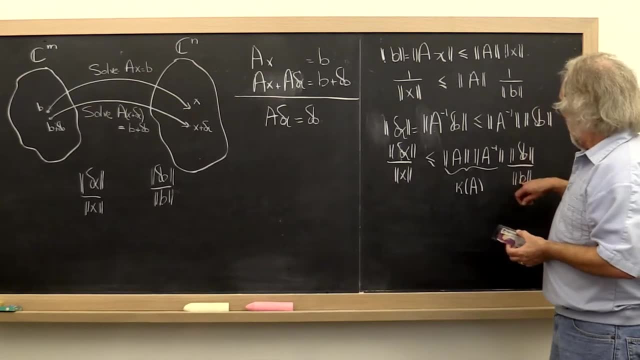 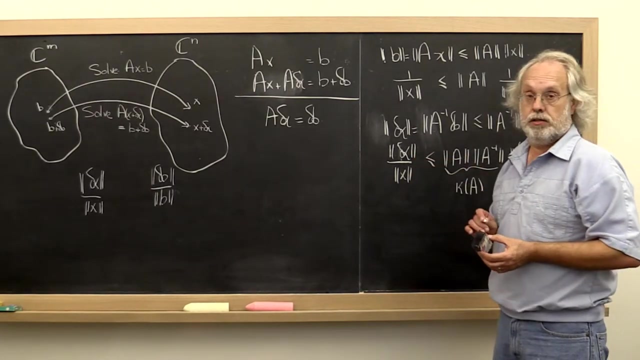 All right. What does that mean? That means that this is a tight bound. This means that there are choices for delta B and B, such that the relative error is actually amplified exactly by the condition number of A into the relative error in x. So this is not a pessimistic view. 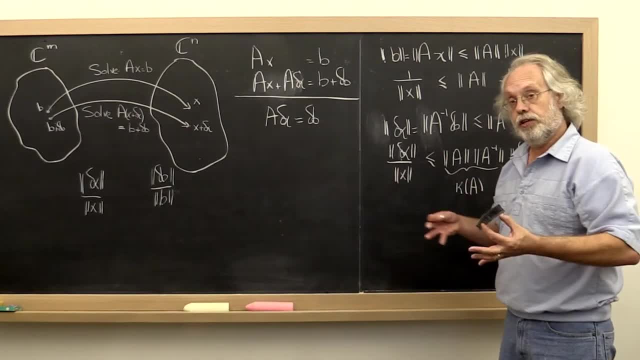 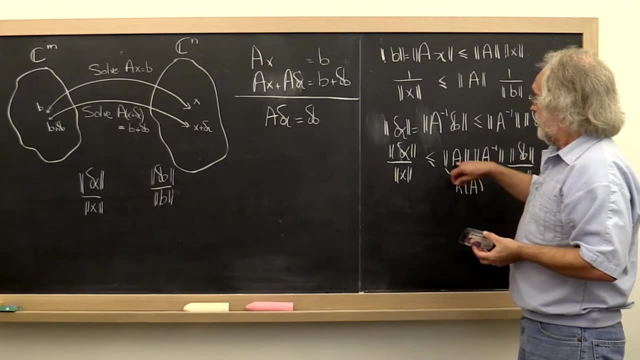 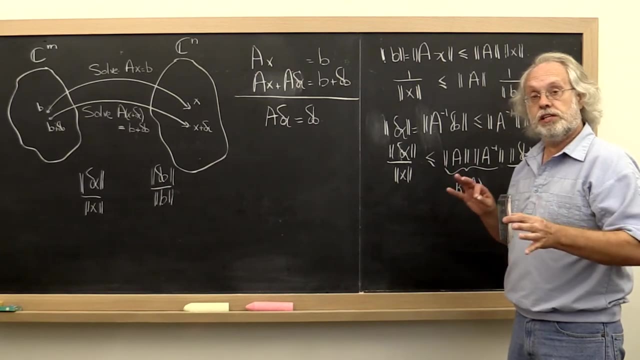 This is something that could happen. Later in the course you're going to find out that the condition number of A depends on how close A is to being singular. So all of these things will start falling in place as we move on through the course. 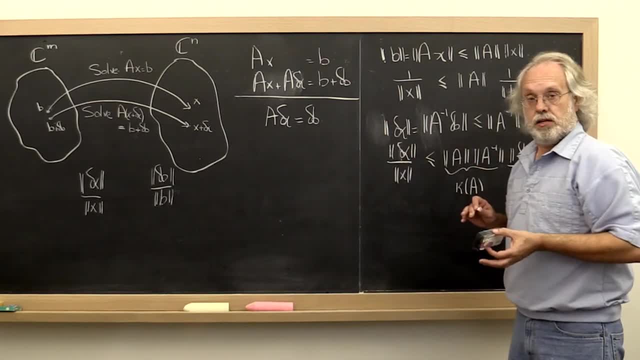 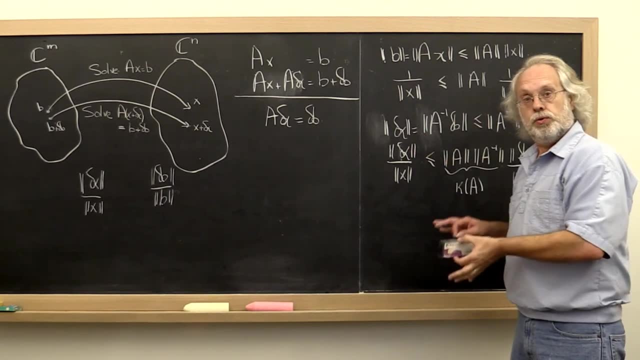 Now in the notes we sharpen all of this, We develop the notation a little bit better, We dot all the numbers, We dot all the numbers, We dot all the i's. We will do a few exercises that will help you along. 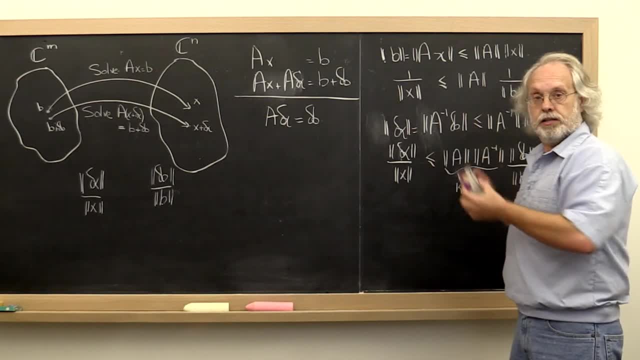 And then you'll hopefully understand everything regarding this topic. 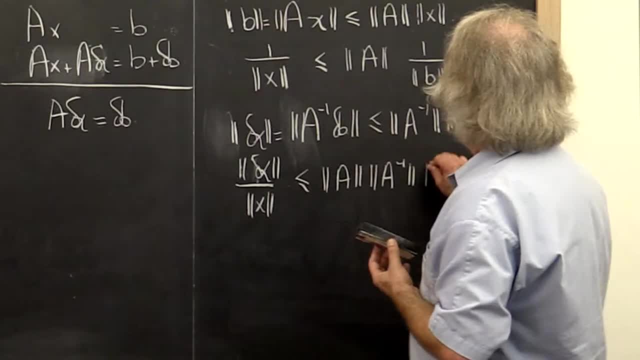 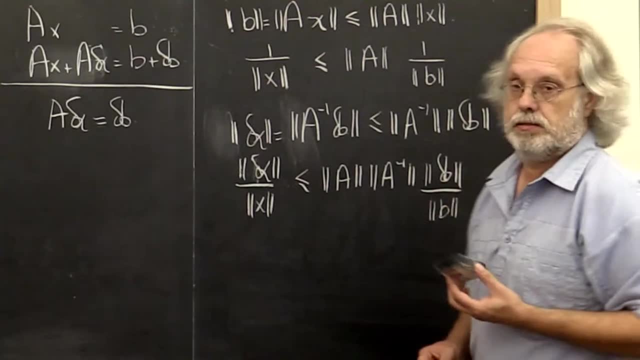 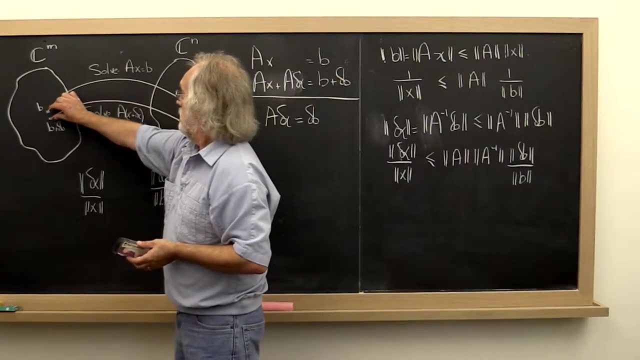 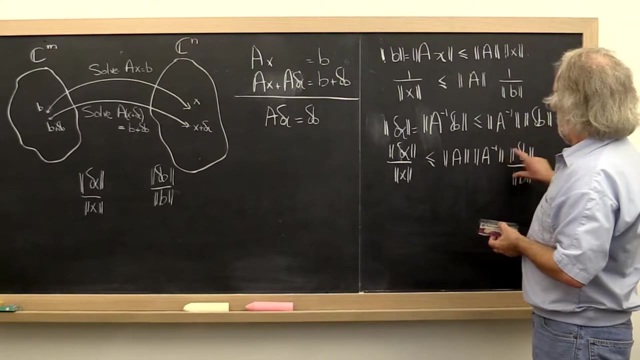 times the norm of A. inverse times delta B, the relative error in B. All right, So we now have answered our question. The small error in B can be amplified no more than this quantity right here, which we call the condition number of matrix A. 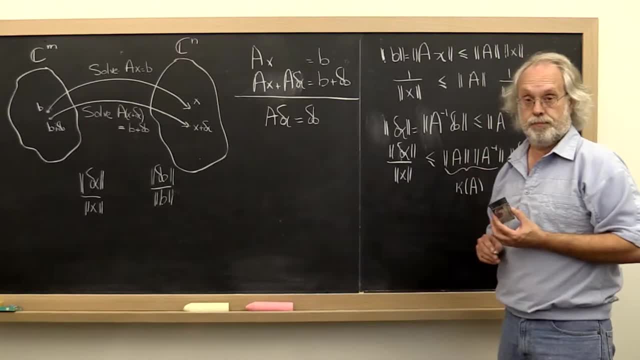 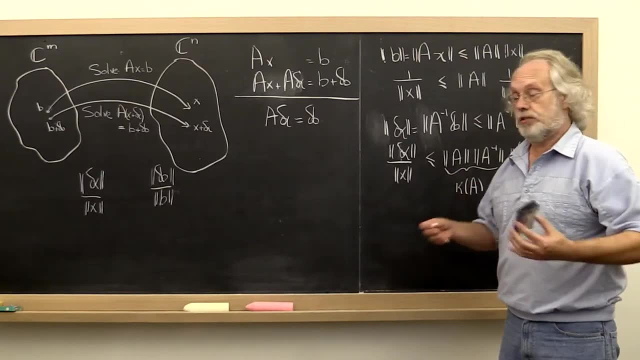 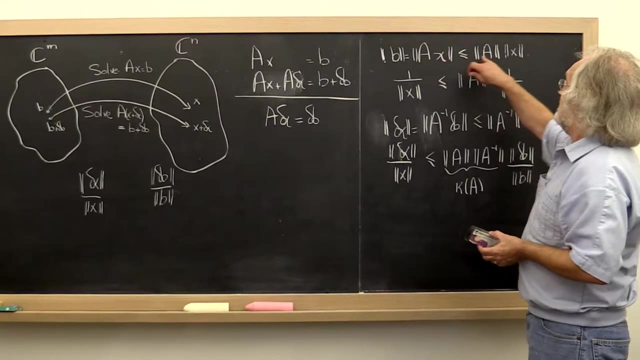 Obviously, this condition number depends on which norm you chose. Now, when we talked about induced matrix norms, we saw that there is a vector x, such that the norm of A times X is equal to the norm of A times the norm of X, And we 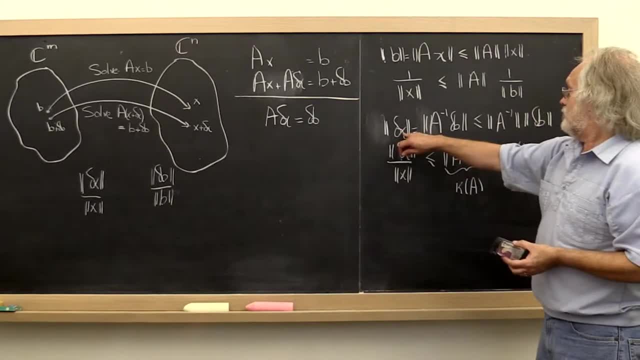 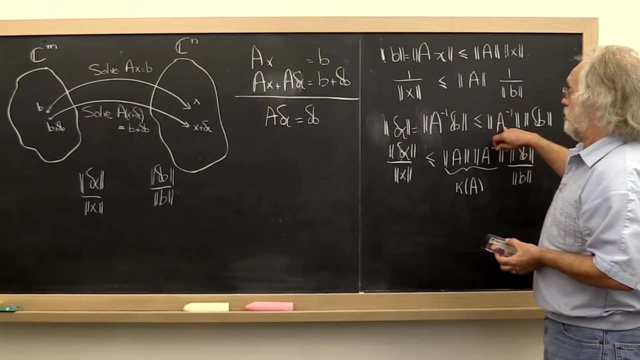 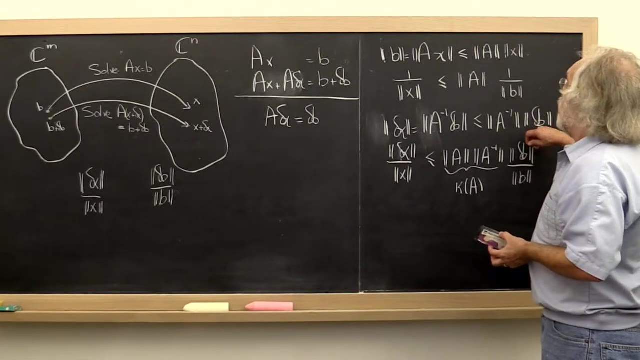 saw similarly that there is a choice for Delta B such that A inverse times Delta B in norm is equal to the norm of A inverse times the norm of Delta B. All right, What does that mean? That means that this is a tide bound. This means that there 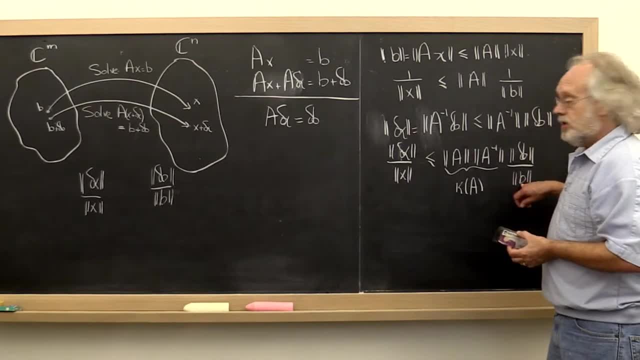 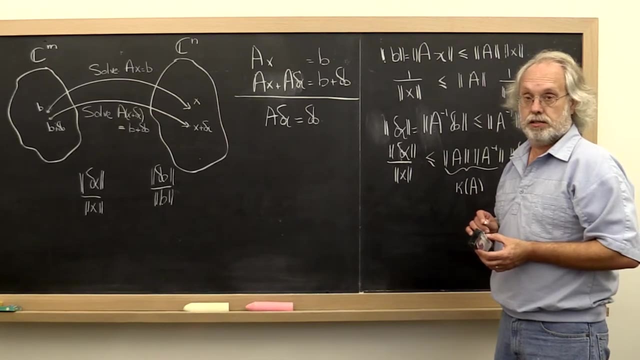 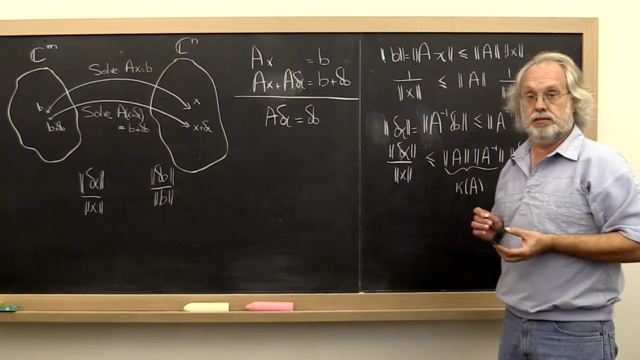 are choices for Delta B and B such that the relative error is actually amplified exactly by the condition number of A into the relative error in X. So this is not a pessimistic view. This is something that could happen Later in the course you're going to find. 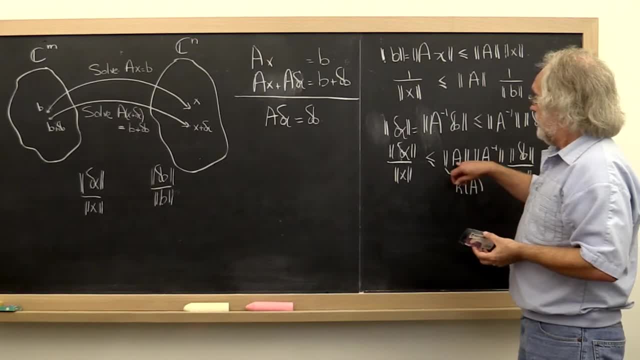 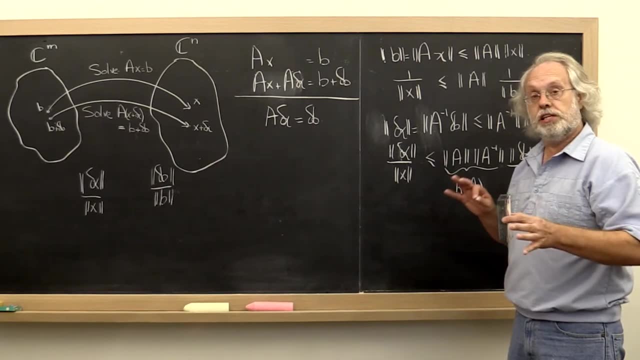 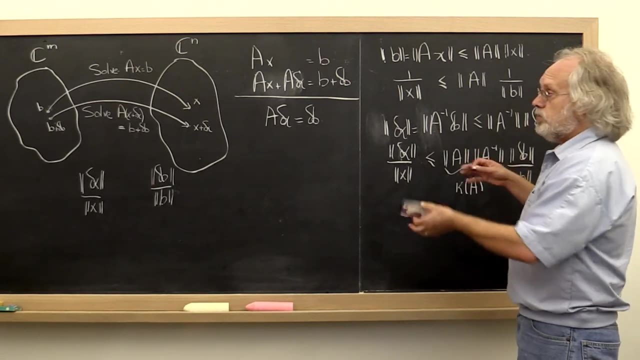 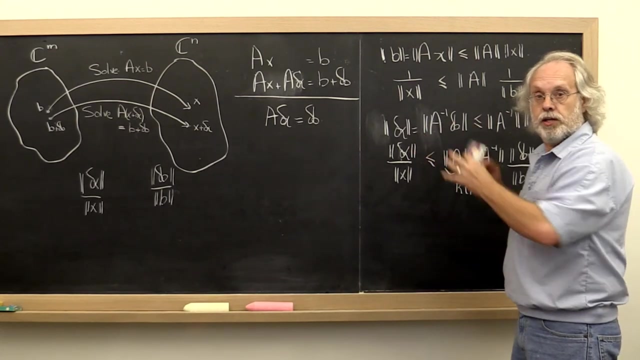 out that the condition number of A depends on how close A is to being singular. So all of these things will start falling in place as we move on through the course. Now in the notes we sharpen all of this, We develop the notation a little bit better, We dot all the i's, We will do a few exercises that. 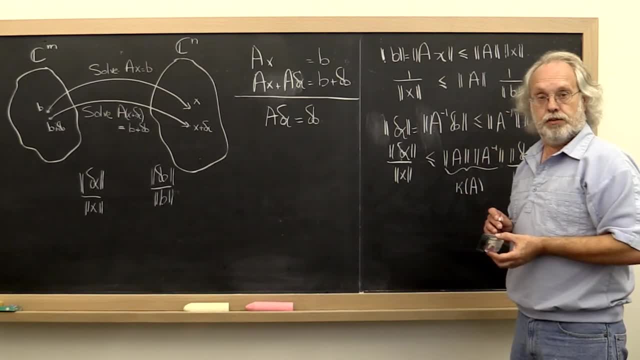 will help you along, And then you'll hopefully understand everything regarding this topic.